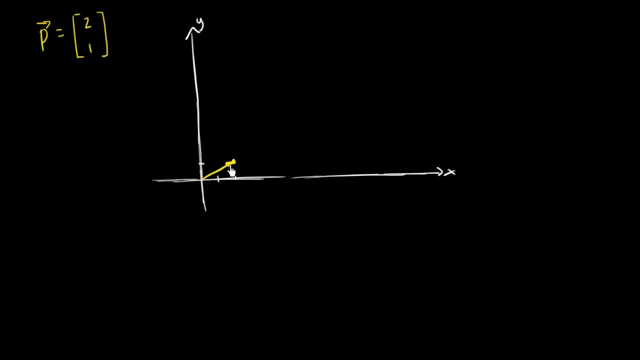 We could represent it in this kind of vector symbol, right like that, where the tail is at the origin and the tip, the head, is at that point. Or we could say it's really representing this position right over here on the coordinate plane. 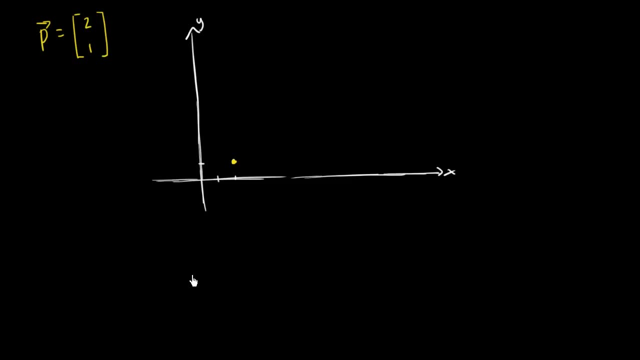 Now, what I want to do in this video is apply a transformation to this position vector, And the way I'm going to do it is: I'm going to multiply our vector p by a matrix, and then the resulting product is going to give me another position vector. 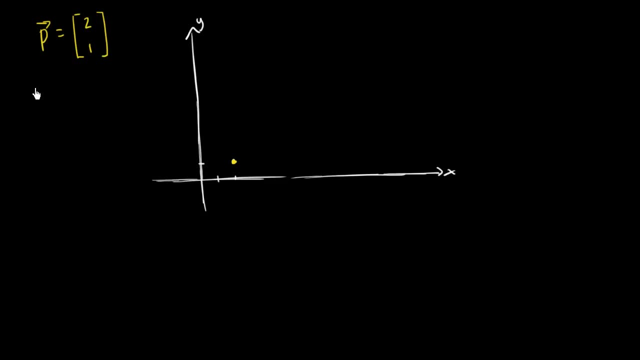 So what do I mean by that? Well, I could have a transformation matrix, capital T, and let's just say it is equal to two. let's say it's equal to two, one negative one and two. So what happens if I multiply t times p? 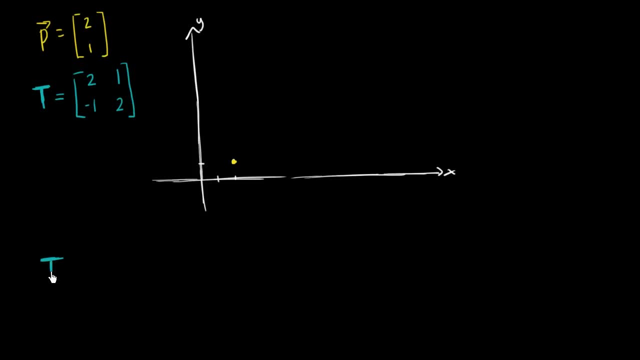 And let's do that right over here. t times p. So first let's just make sure that this is actually a valid operation, that matrix multiplication or matrix vector multiplication is defined here. So let's just look at what t and p look like. 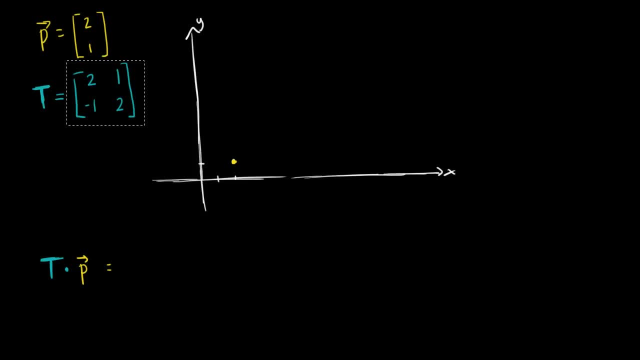 We already know what they look like, so I'm going to copy and paste. Copy and paste. That is t and this is p, right over here. So copy and paste And let's see. can we multiply a two by two matrix? 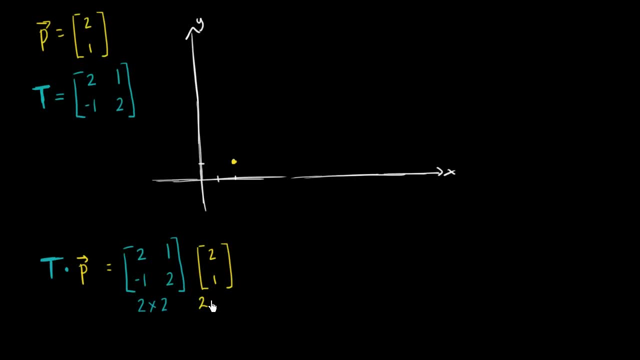 times a column vector like this, which is essentially a two by one matrix. Well, sure as we know, matrix multiplication is only defined- or at least a conventional matrix multiplication is only defined if the first matrix, the first matrices, number of columns. 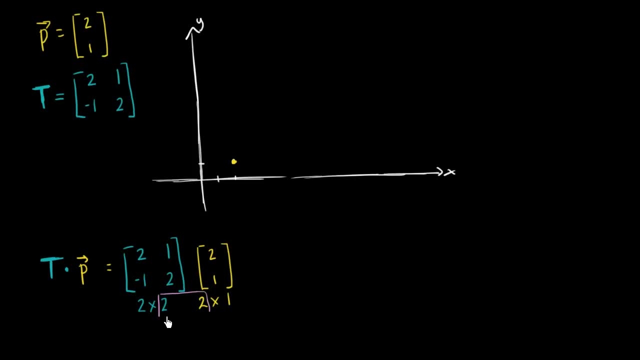 number of columns is equal to the number of rows in the second matrix right over here And we see both of those are two. So this is going to result in a two by one matrix. So this is going to result in a two by one matrix. 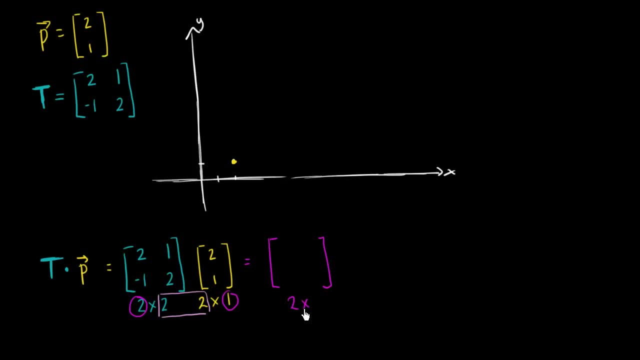 Now what's interesting about that? what's interesting about that is that this is another column vector, this is another position vector. So you took this vector p, multiplied it by this transformation vector and we're going to get another two by one.